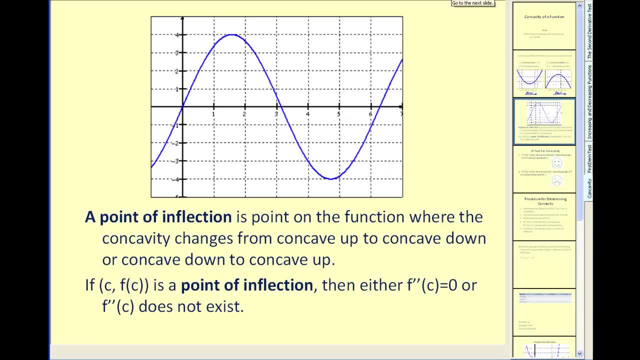 like an upside down cup Putting those pieces together. if we look at this graph, we can see that it's concave down and in this interval over here it's concave up. Somewhere in the middle here it changes from being concave down to concave up. That point has a special 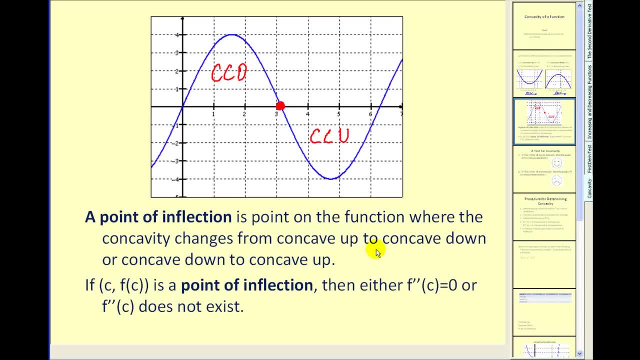 name. it's called the point of inflection. A point of inflection is a point on the function where the concavity changes from concave up to concave down or vice versa. If c, comma f of c is a point of inflection, it's concave up. 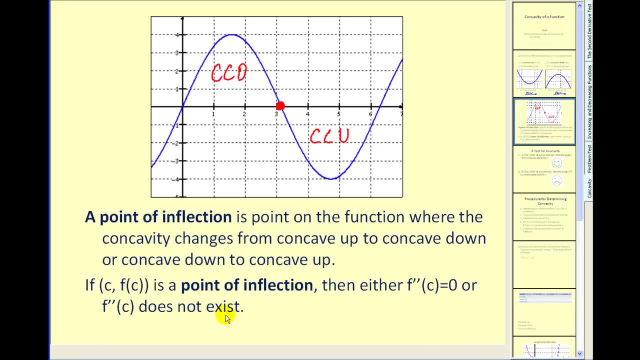 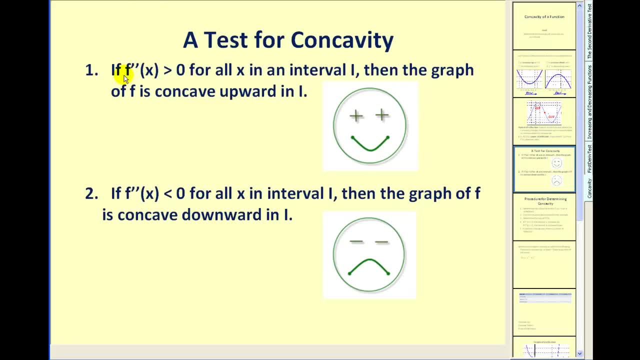 Then either the second derivative is equal to zero or the second derivative does not exist. Here's an easy way to remember the test for concavity: If the second derivative is positive or greater than zero on an interval, then the function is concave up on the interval. 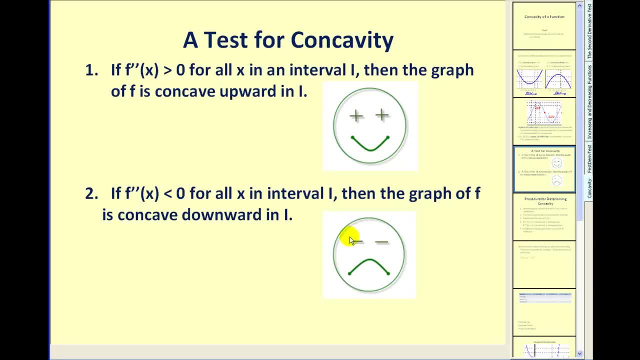 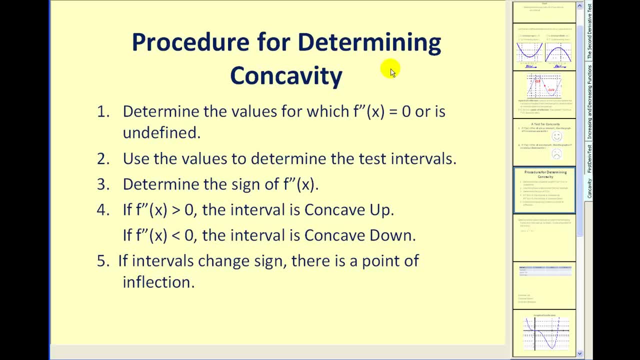 If the second derivative is negative or less than zero on the interval, then the function is concave downward. Let's put all these pieces together. Here's the procedure for determining concavity. Step one: we will determine the values for which the second derivative is equal to zero or 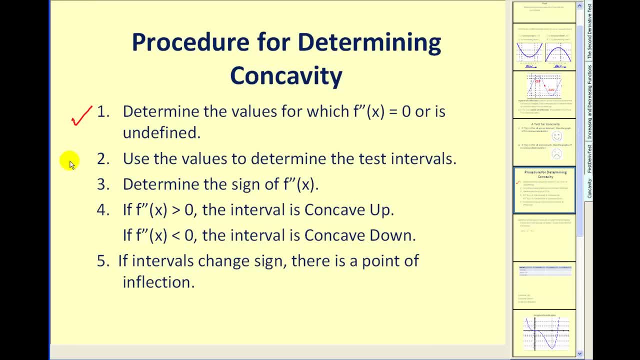 undefined. Step two: we'll use these values to determine the test intervals over the function's domain. Then we'll determine the sign of the second derivative, As just stated. if the second derivative is positive, it's concave up on the interval. If it's negative, it's. 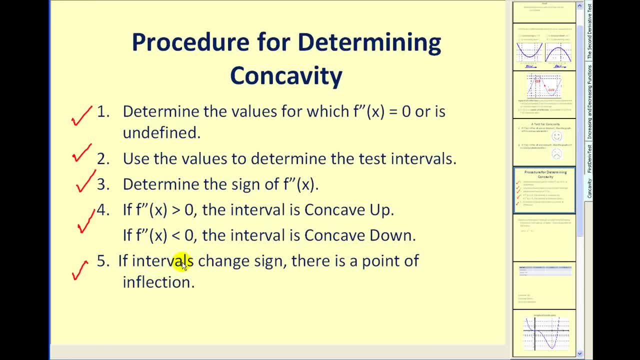 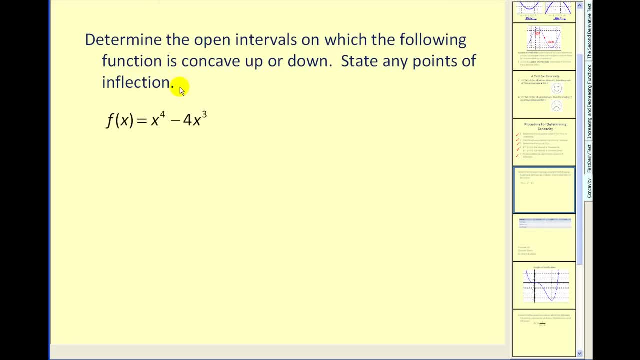 concave down. And last step: if the intervals do change sign there is a point of inflection. Let's go ahead and give it a try. Determine the open intervals for which the following function is: concave up or down. So we have to figure out where the second derivative is equal to zero. We first find: 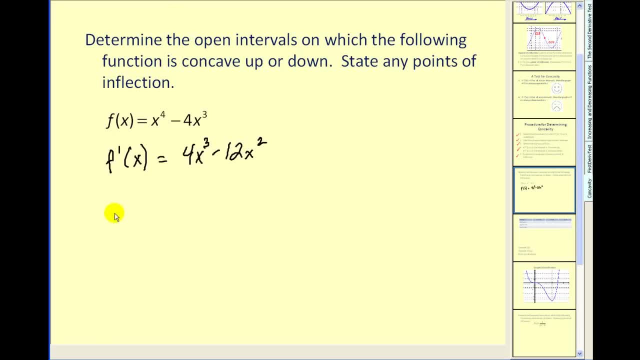 the first derivative. Now we find the second derivative. There are no values of x where this is undefined, so we set it equal to zero. Step 3, we'll empty the first derivative into polities, But only step 1 is an empty. 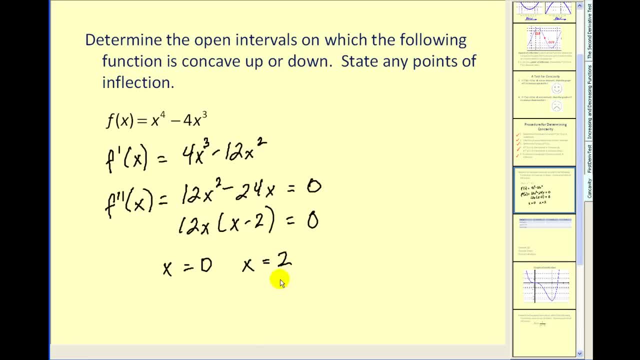 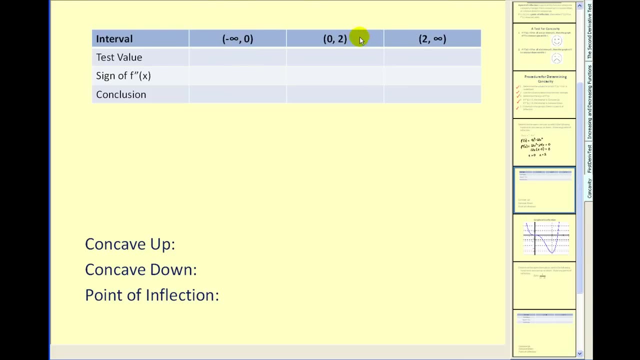 囧. Step 2, we find the first derivative right under the first interval itself is athlean. Step 3, we'll differently new the estoin. Let's call it now the 2 INS. Step 4, we'll nearly confuse the 2 INS. 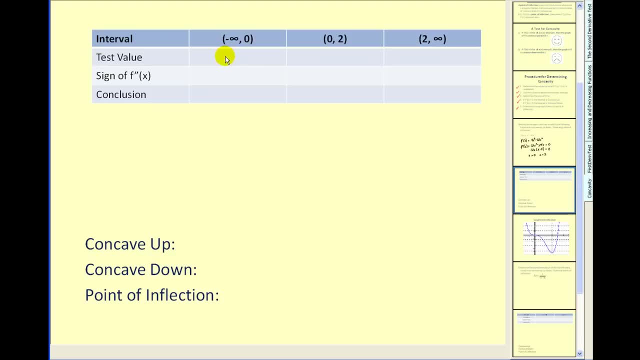 Now to take those weghts. we're going to take norm derivative test, which tests for increasing and decreasing. But because we're dealing with the second derivative now, we're testing for concavity, So we'll pick our test values. 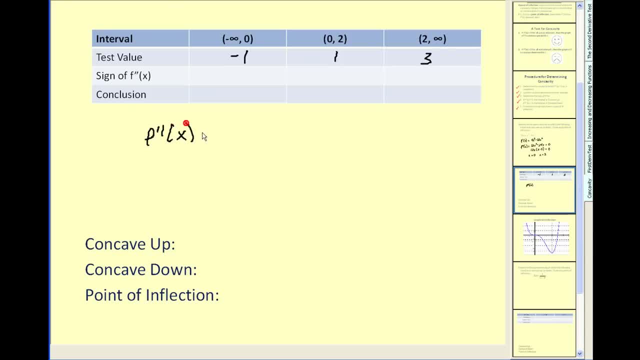 And what we'll do now is type our second derivative into y one and use our calculator to evaluate the sign of the second derivative. Remember, the second derivative was equal to 12x squared minus 24x. Let's go to our graphing calculator. 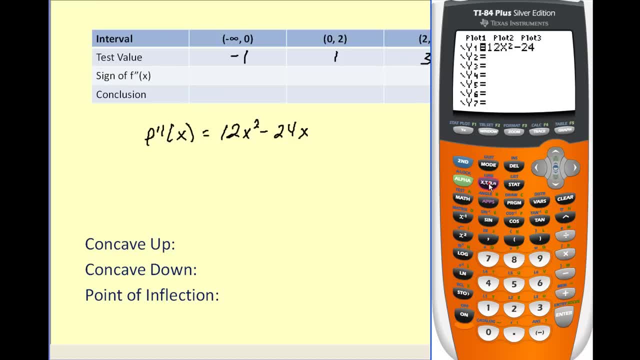 and type that into y one. Let's go to our table feature And we're going to test the sign at negative one, one and three And we can see: first interval is positive, then negative, then positive. Let's go ahead and record this. 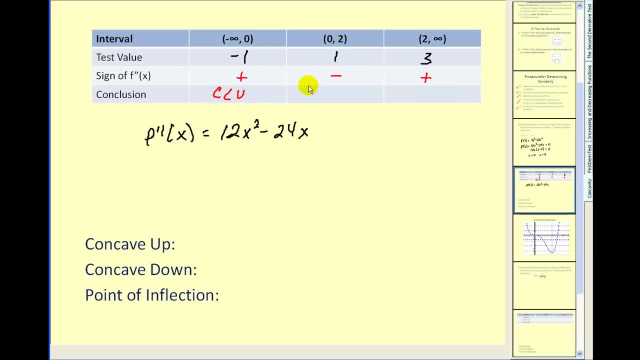 So what this tells us is the function is: concave up on this interval, concave down, Concave down on this interval and concave up again on this interval. Since it does change concavity, we do have a point of inflection at zero. 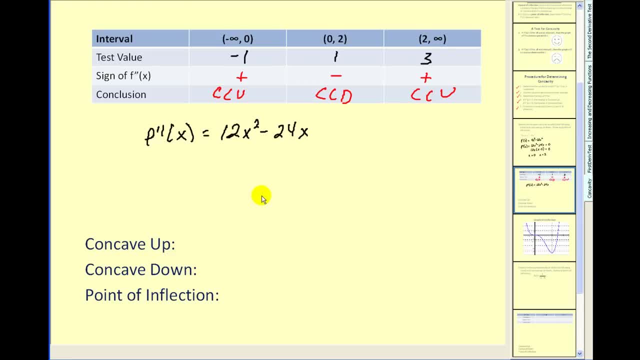 and also at x equals two. So let's go ahead and record this information. We have a point of inflection: when x is equal to zero, We still have to go back and find the y coordinate of that point. And we have another one at x equals two. 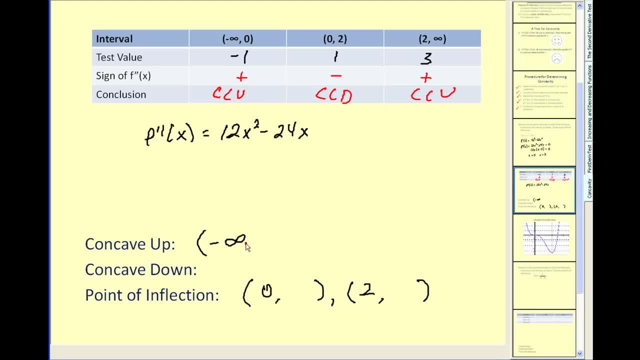 We said, it's concave up from negative infinity to zero And from two to infinity, And it's concave down from zero to two. Okay, so, lastly, we have to evaluate the function at x equals zero and x equals two. Remember our original function was f of x is equal to. 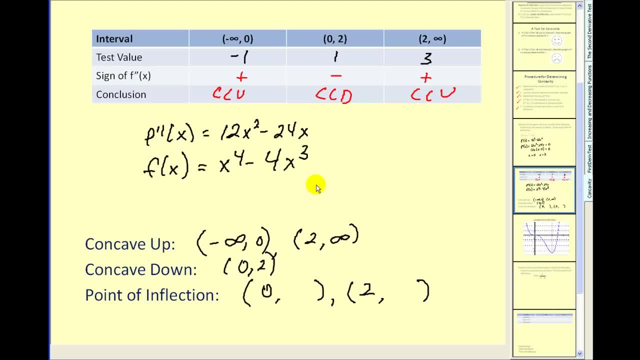 x to the fourth minus four x to the third. Well, we can easily sub in zero for x and get zero for y. Let's go ahead and find f of two. Two by hand Looks like we would have 16 minus 32, which is equal to negative 16.. 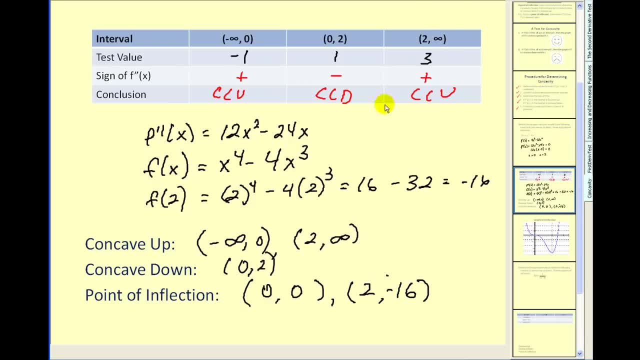 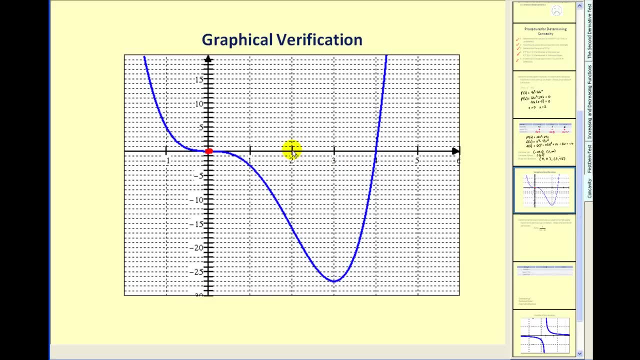 Okay, so let's go ahead and test all this information that we found by analyzing the graph. First, we found a point of inflection at zero. zero and two negative 16.. On this interval, it's concave up. On this interval, it's concave down. 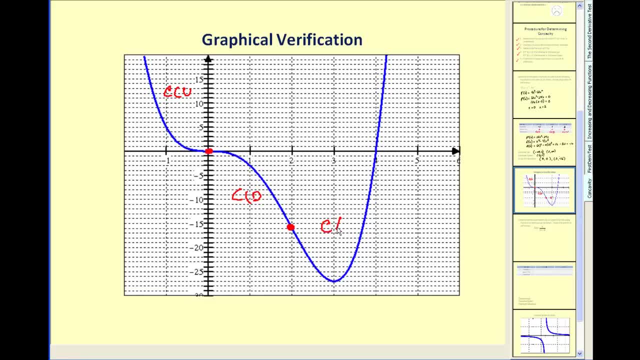 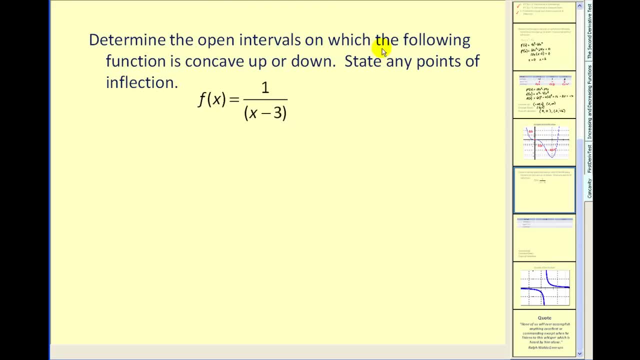 And the remaining interval it's concave up. again, This verifies our work. Let's try one more. Determine the open intervals on which the following function is concave up or down. State any points of inflection. Okay, so we have to find the second derivative. 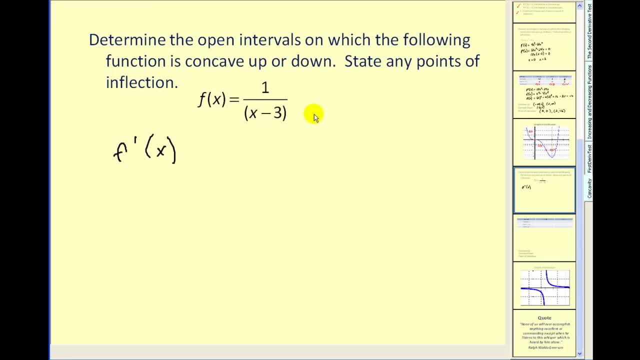 of this function. So we find the first derivative. Now, out of the two, we have to find the second derivative. By the way, you may think quotient rule, but we can rewrite this as the quantity of x minus three raised to negative one power. 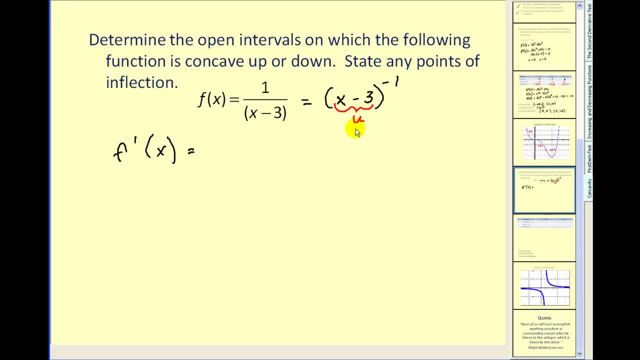 So we'll go ahead and apply the power rule. So we'd have negative one u to the negative, two power times u prime. but u prime is equal to one in this case. So our first derivative simplifies to this. Now we need to find the second derivative. 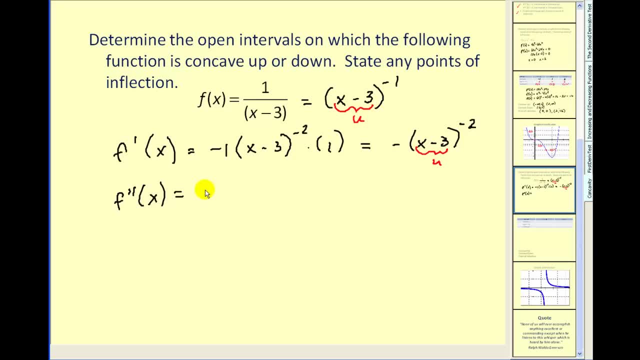 Again we'll apply the power rule. So we'd have two times the quantity x minus three raised to the negative third power times, u prime. but again u prime is one. So our second derivative is equal to two divided by the quantity x minus three. 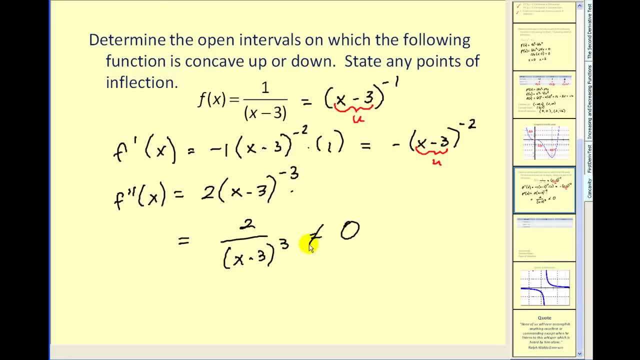 raised to the third power. Now, this will never equal zero, but the derivative does not exist when x equals three, And in fact x equals three is also a point of discontinuity, And in fact x equals three is also a point of discontinuity.